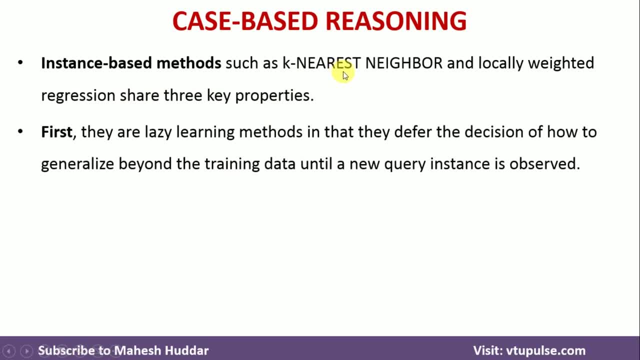 is, these methods, like k-nearest neighbor and locally weighted regression algorithms, are lazy learning methods. That is, unless and until we get a new query instance, these methods will not do any learning. Whenever we get a new instance, we will use the training. 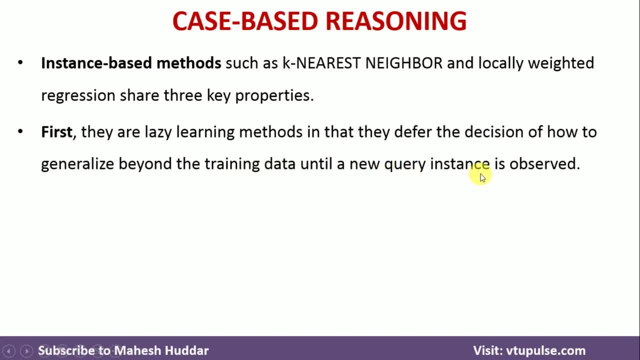 data and then this new instance will be classified based on either the nearest neighbors or, you can say that, locally weighted nearest neighbors in this case. I have discussed these two algorithms in detail in the previous videos. the link for those videos is given in the description below. There you will understand how these particular 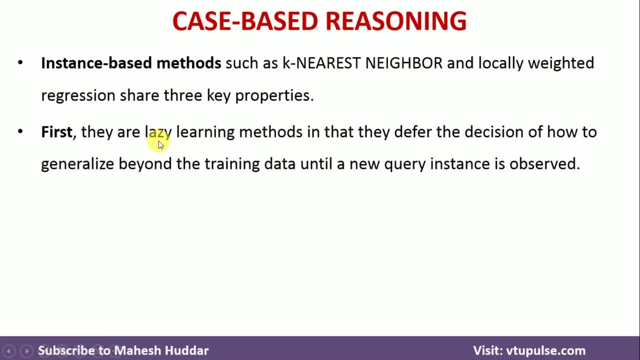 algorithms will work and why they name given like lazy learning or something like that. The second one is they classify the new instance by analyzing the similar instances, that is, when it comes to k-nearest neighbor or locally weighted regression algorithms. they consider only the nearest examples to classify the new instance. 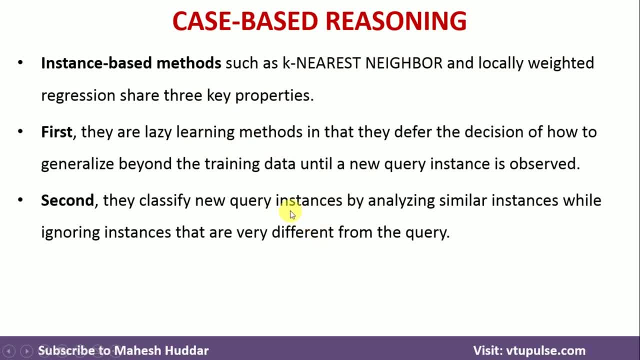 they will not consider all the instances which are present in the training data. they consider only the nearest instances. so that is the another property of this instance based methods here the third one is each and every data in this kind of methods is represented as real valued points. 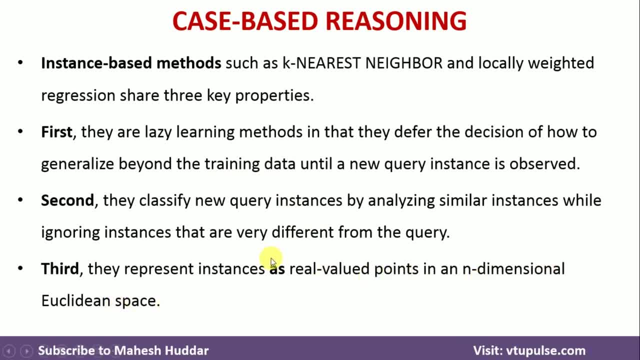 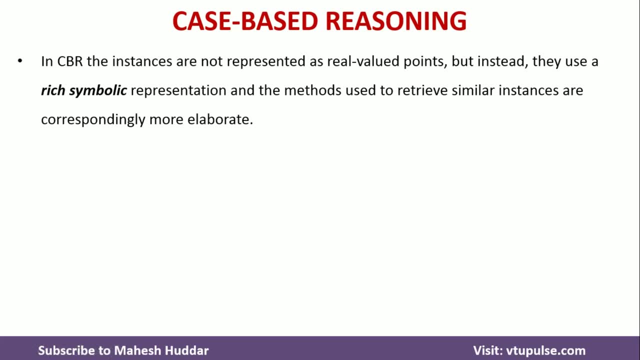 in a n-dimensional euclidean space, that is nothing, but everything is a real valued in the form of table or something like that. that is the another property of this particular instance based methods. now, coming back to this, case-based reasoning or case-based learning methods, in this case, 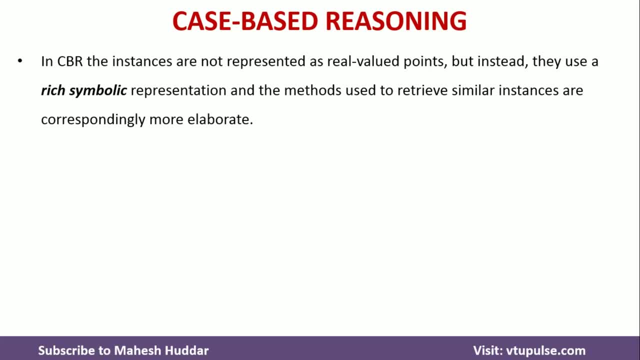 we don't represent the data in the form of real valued points or something like that. what we do in this case is we will use something called as a rich symbolic representations of the cases, you can say, and the methods used in this case are the ones which are represented as real valued points. 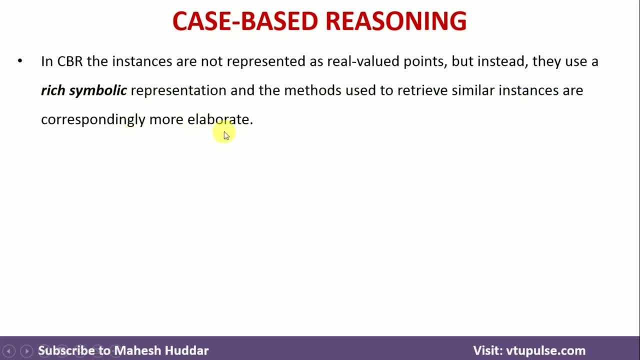 to retrieve. similar instances are correspondingly more elaborate over here, so now we will consider few examples. to understand how cbr will work, let us say that we are trying to design a mechanical device. so what we do here is, in this kind of cbr method or case-based reasoning method, we store 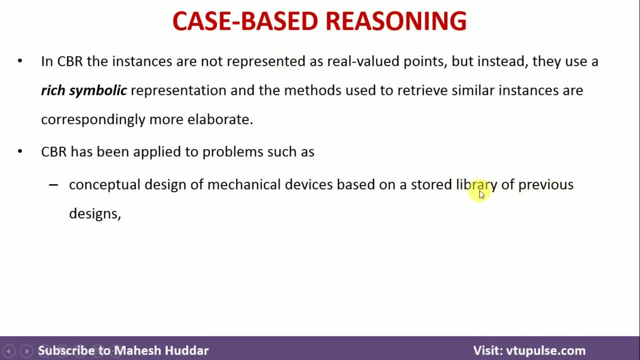 a previous design in the form of a library. whenever you want to design a new mechanical device, we will go through those particular previous designs and then we will try to match the previous designs with a new requirement. if any of those previous design matches with a new requirement, we will consider that particular. 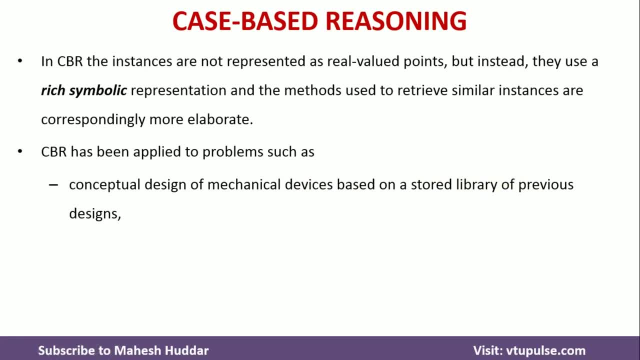 design and then that will be given to the customer. if customer is happy with that particular design, yes, it's the final one. otherwise, if the customer is not happy, what we need to do is we need to do some modification and then that thing should be given to the customer over here. so that's how this. 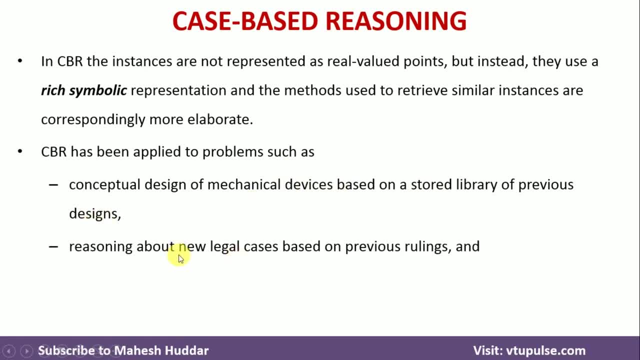 will work. take another example. let us say that you are trying to solve a legal case. so what we do in this case is we will consider the previous rulings as the cases, so we will match the new legal case with the previous rulings. the one which will match with the previous ruling we will consider. 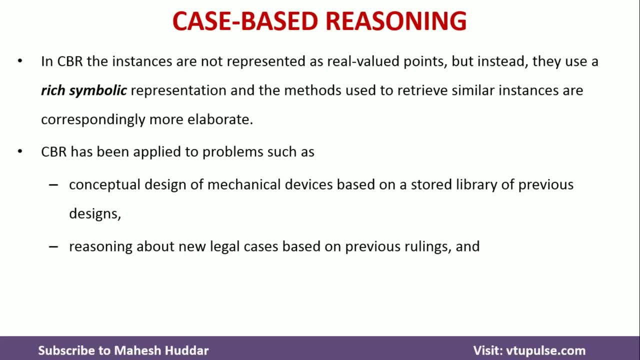 if there is a slight modification is required again, we will do the modification and then we will apply that particular previous ruling to the new case so that there is a maximum possibility of that particular case or something like that. now we will try to understand what are the different. 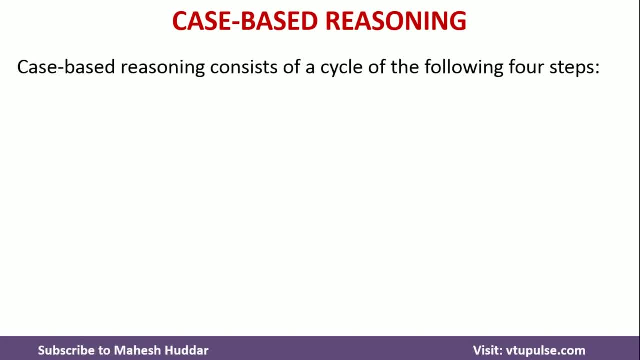 steps to be followed in case based reasoning technique. the first step is retrieve. given a new case, we need to retrieve the similar cases from the case base. we must be having some library of cases. we need to match this particular library of cases with the new case, the one which is more 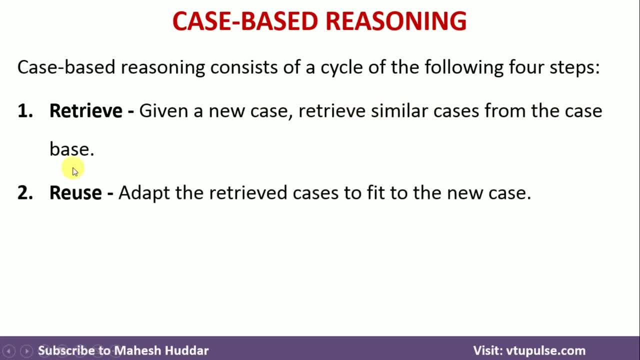 similar, we need to retrieve it. that's the first step. once you retrieve that particular thing, we need to check whether that particular solution is exactly same or there is a need of some modification with respect to new case. if it is exactly same, there is no need of any modification. 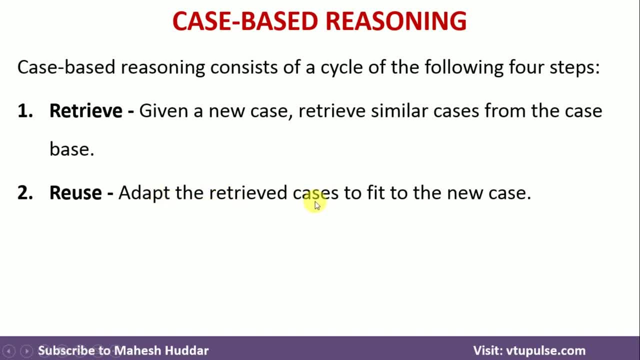 if it is not exactly same, we need to do some modification so that it will fit to the new case over here. so that's the second step in this case. the third thing is, once you apply that particular existing case with to the new case, we need to evaluate that particular. 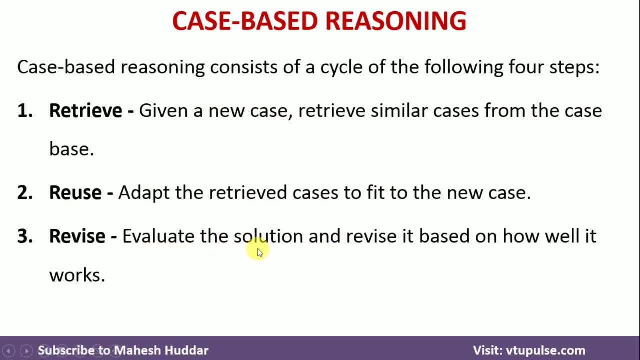 solution whether it is working fine or not. if it is working fine, then it's okay. if it is not working fine, again, we need to do some modification to that existing case so that it will work perfectly fine on the new case over here. the fourth one is very interesting. if you have not done any modification. 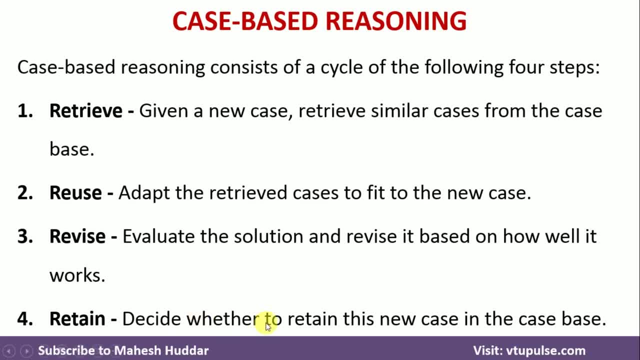 the fourth step will not come into picture because you already the case is present in the case base, so there is no need to retain it or store it again. but if you have done some modification to that case you have extracted from the case base, we need to make a decision whether to retain that particular. 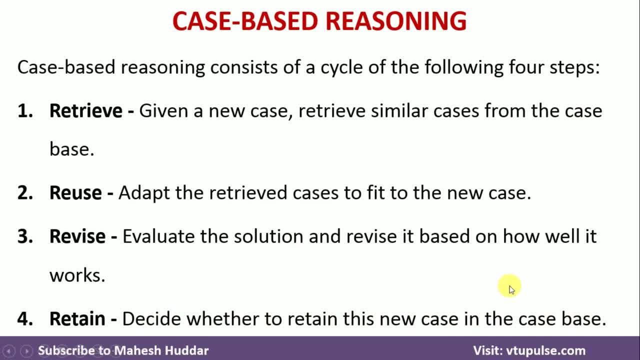 new case in the case base or we should not retain it. so that is the decision we have to make. but here we can make a decision based on whether we have done some modification or whether we have not done modification to the existing case. if you have not done any modification, there is no point in. 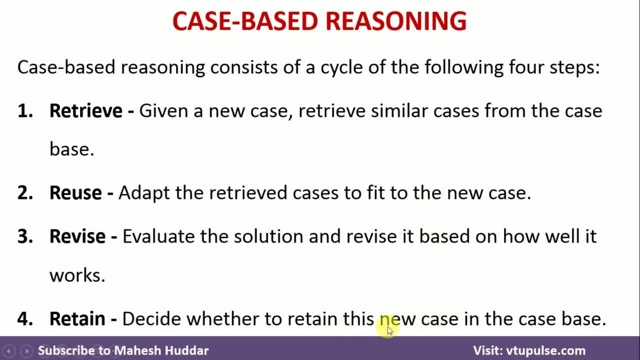 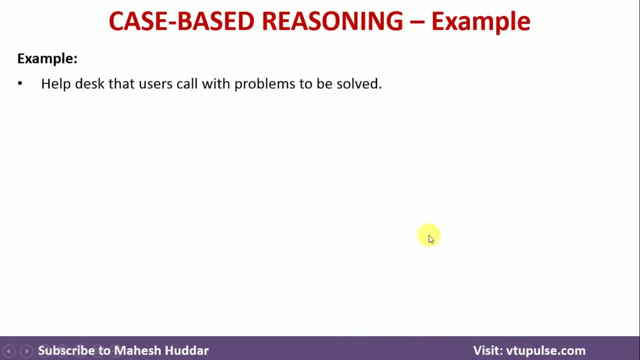 storing the new case here. if you have done some modification, definitely you have to store the new case into the case base over here again. we will take one more example to understand this one. let us say that there is a help desk where the customers will call to get some solution to their problems. okay, so what actually happens is whenever they call. 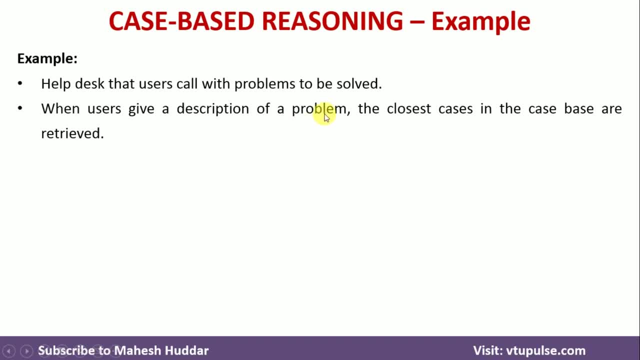 they will give the description of that particular problem. so what the help desk person will do is they will search for the closest case, what they have solved or what they have suggested to the customers. once they get that particular closest case, they will recommend that particular closest to the user. for example, let us say that the person will call to the help desk and they 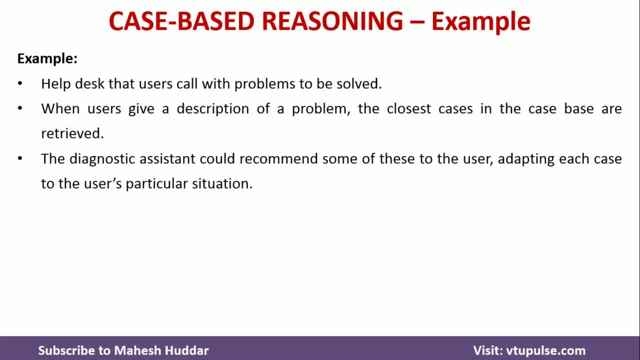 say that the internet is not working in my mobile. so whenever this description is given to the help desk person, they will search the closest case to that particular description and then they will recommend the solution. so it may happen that the solution may work or it may not work. if it works, it's fine. if it doesn't work, what we need to do is we need 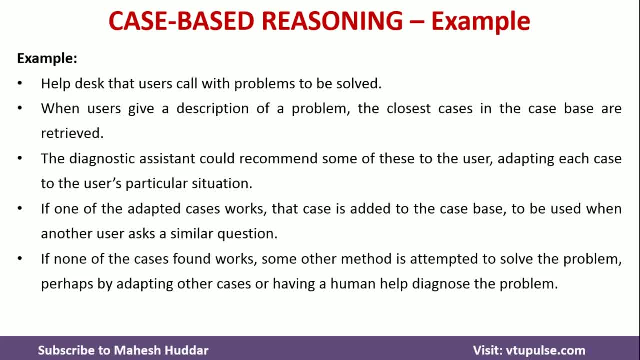 to give some other solutions and so on. so that's how actually the thing will go on. go on over here. if the existing solution is working, there is no point in storing it into the case base. if it is not working and if you have suggested some new solution, you can store. 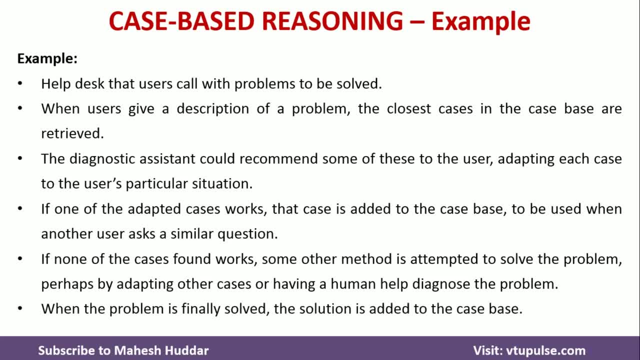 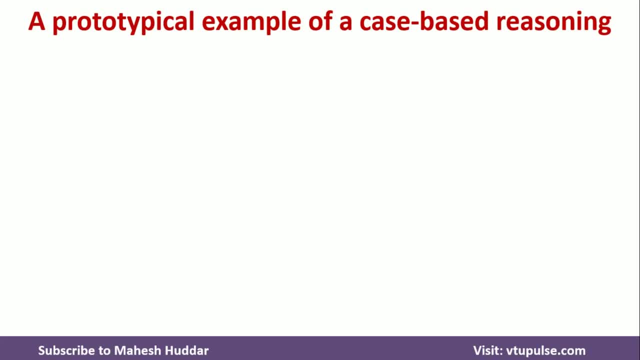 that particular thing into your case base and so on. so that's a very simple idea behind this particular case based reasoning algorithm over here. now one more example we will try to take so that we can get a clear picture of case based reasoning here. let us say that we are trying to design a mechanical device such as water. 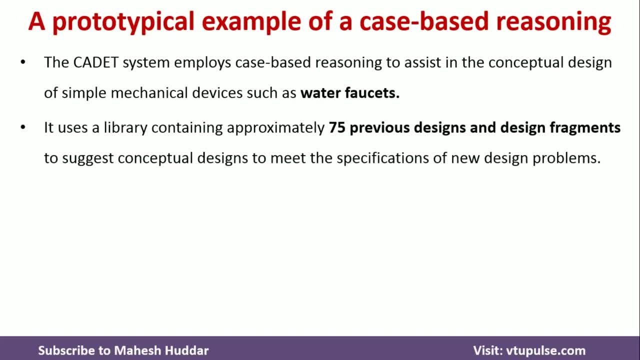 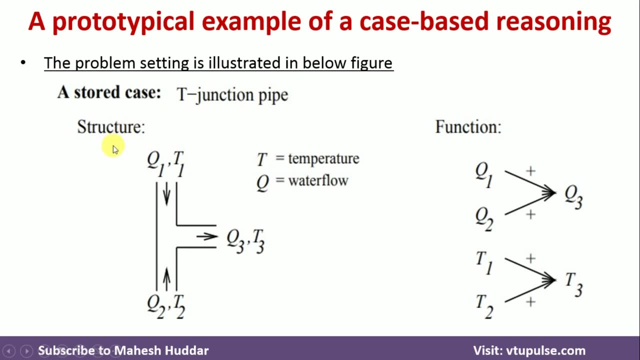 facets. what we can do here is we can create some designs. let us say that 75 designs were stored into the database, that they look something like this one they are. they will have two things: one is structure and another one is function: the structure of that particular faucet and what is the functionality of that particular faucet over here. so it is a. 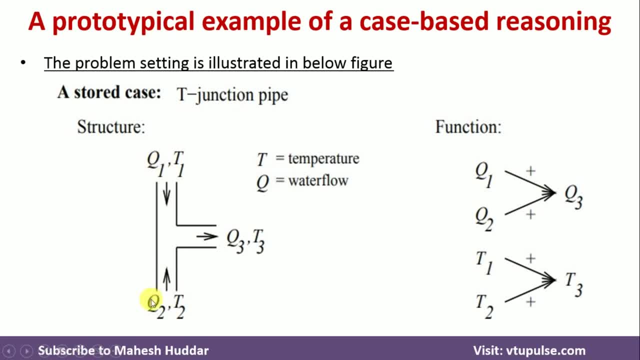 t junction pipe, where q1, q represents the water flow and t represents the temperature here. so water is flowing in this direction and it is flowing in this direction. so the functionality over here is q3 is equivalent to what q1, q2. so because both are coming in this direction only, 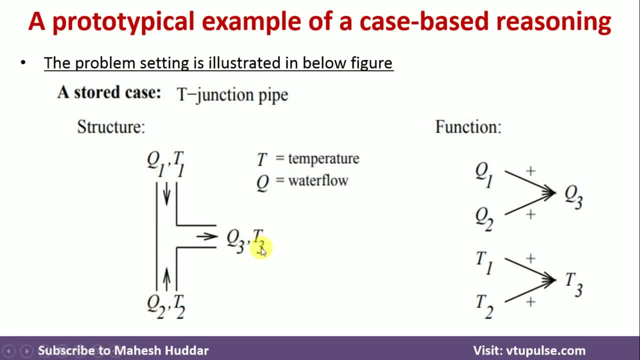 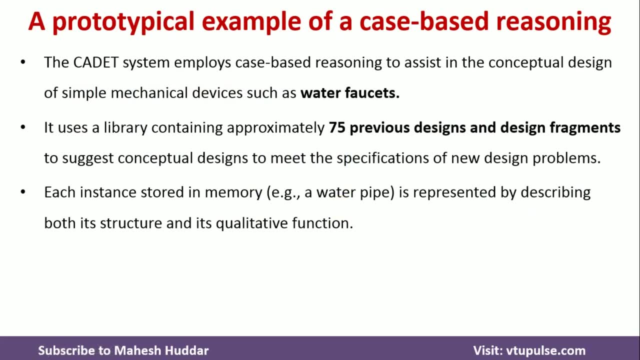 so q3 is equivalent to q1 plus q2, t3 is equivalent to t1 plus t2, and so on. so this is how. what we do is we will store the previous designs whenever a customer comes to us, and then they will give the problem description or what they are expecting in water faucets or something like that. we will. 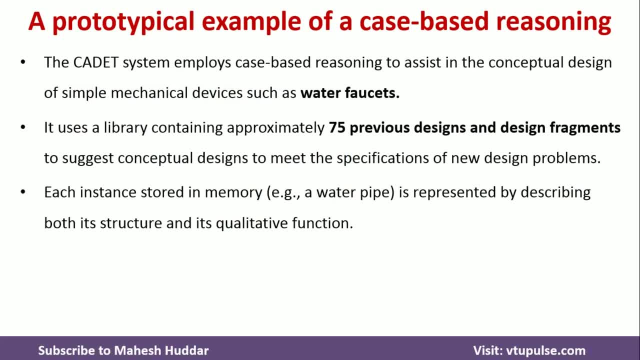 retrieve one of this particular design based on his description, and then that will be given to the customer. the customer may be satisfied with the design and then he will give the design to the customer and then he will give the design to the customer and then he will give the design to the customer. 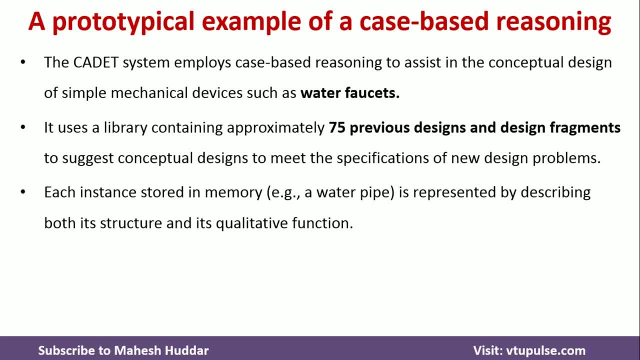 with that particular solution, he may not be satisfied. if he has satisfied with the given solution- yes, that's the final one, because already available- we have presented the same solution to the customer. if he has not satisfied, we need to do some modification to that particular design and then we need to present it to the customer over there. so, because you have done some modification, 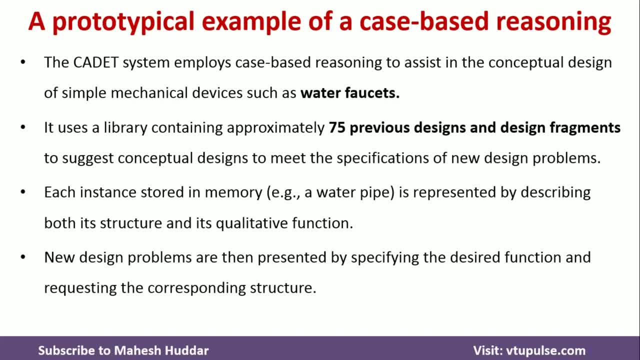 you can store that particular new design and it will become the 76th design and so on. so that is how actually the case-based reasoning works in this case. so in this video i have discussed how to apply case-based reasoning in machine learning. with a simple examples, i hope the concept is clear.